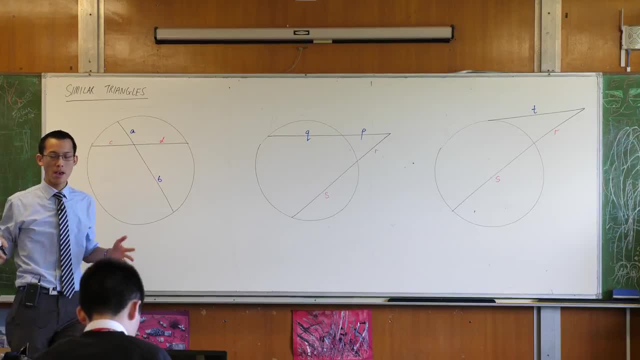 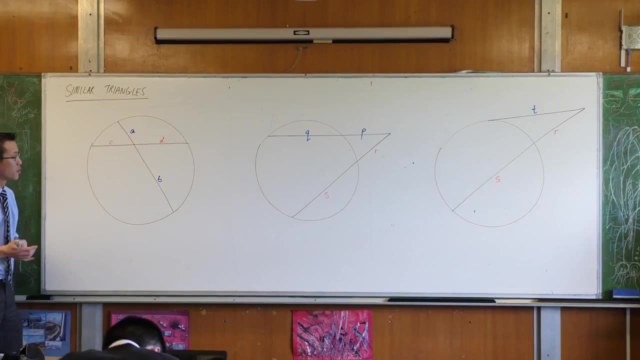 right. When we proved that, do you remember? I said you had to make a construction and I said: whenever you're making constructions, you don't know where to go. a good idea is to put the centre on The reason. why is that once you've got the centre there, it is you. 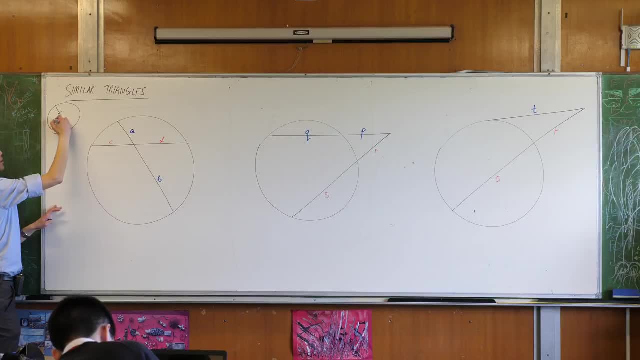 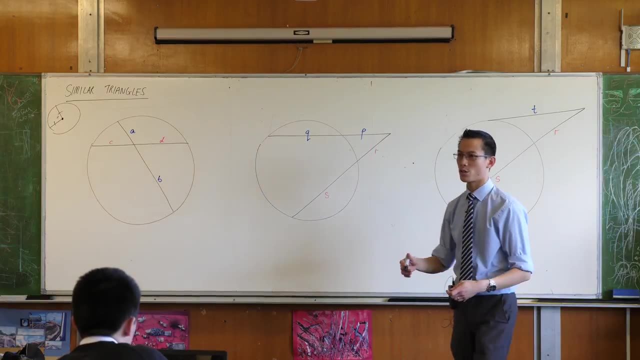 have all kinds of equal lengths because of all of these radii here and you can take advantage of those, because equal lengths give you lots of isosceles triangles. isosceles triangles give you equal angles and you can get lots of stuff from that. 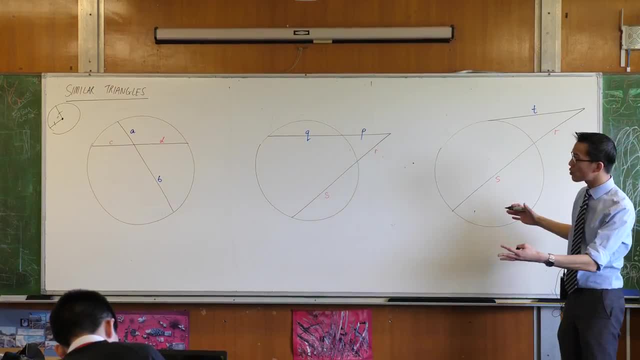 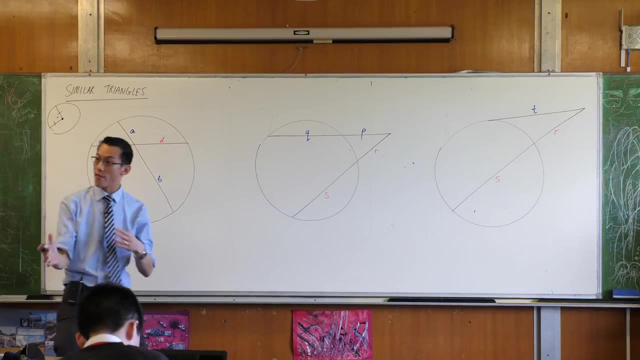 Now, in addition to that, we're going to talk a little bit about what we're going to do next. In addition to isosceles triangles, circles also create a bunch of similar triangles. they come up everywhere Because there are so many angles that are equal. when you have 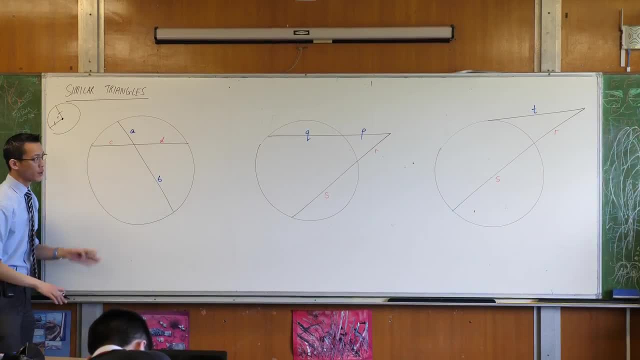 angles that are equal, you get similar triangles. So I'm going to show you three sets of similar triangles here, each of which gives us a really nice property about the intercepts in these circles. So here's the first set up over here. you can see I have a pair of. what are these? 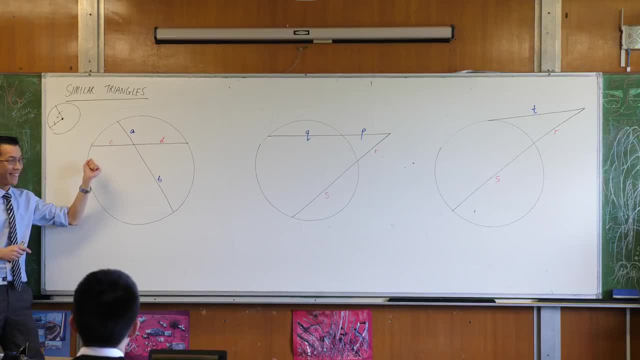 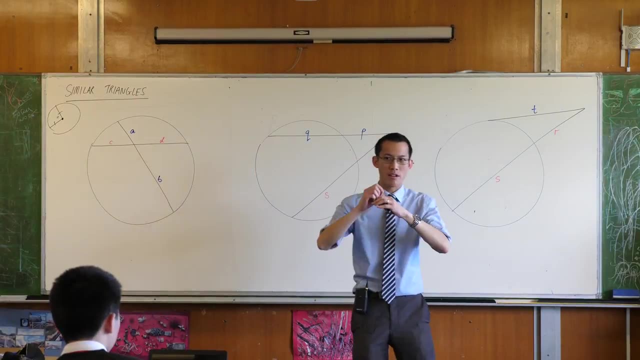 shapes on the inside of the circle. what do you call them? They're chords, right chords, and because they clash, we call them intersecting chords. They're not just chords that are out there randomly, they have to touch in order to get this kind of configuration. You can. 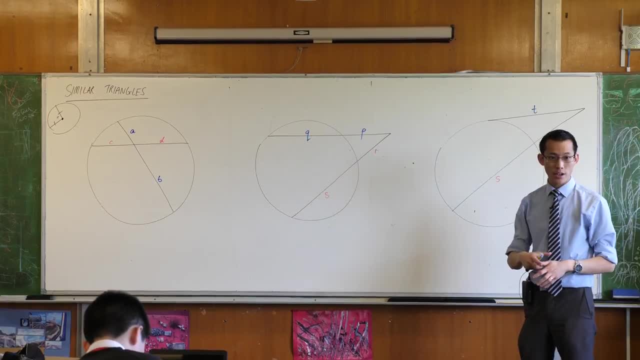 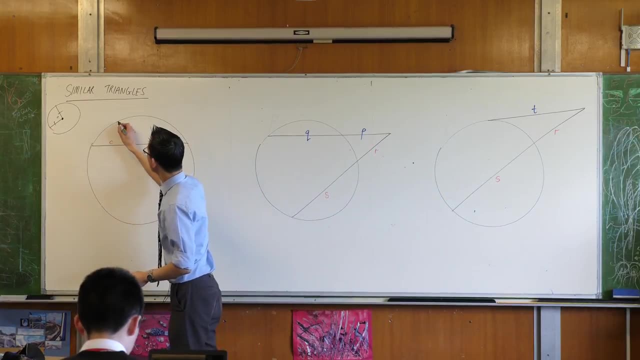 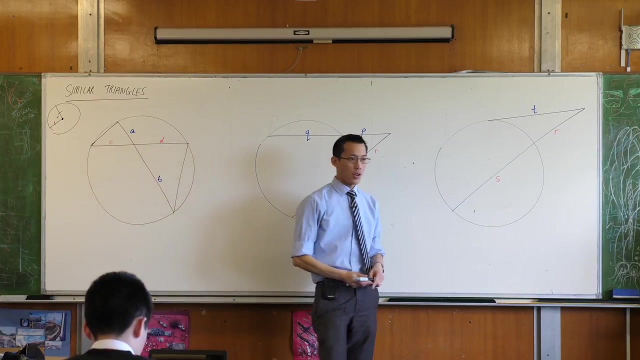 clearly see that they create similar triangles. if you just join up some of these chords, so you can do this in more than one way, but I think for me the most obvious way is along that edge, up the top And also down here. So it might not be immediately apparent to you that these are similar, but 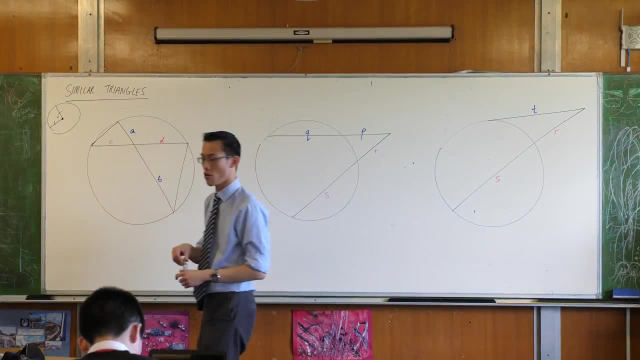 it's not hard to see what's going on, right. Think about some properties that you know already. I know I don't need to- I'll just stay with black- And I want you to tell me where some angles are that we can use to prove similarity. I only need two pairs, Sean give. 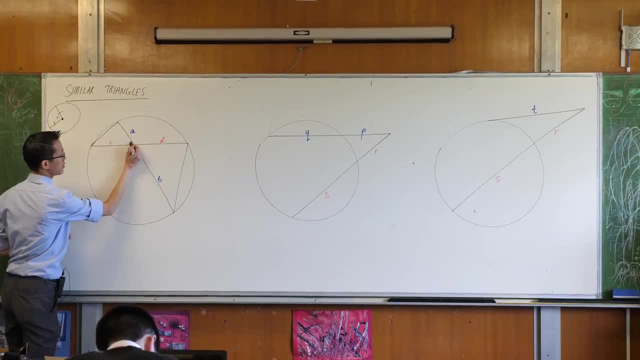 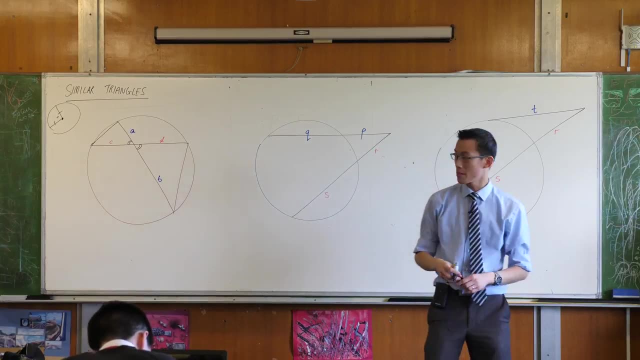 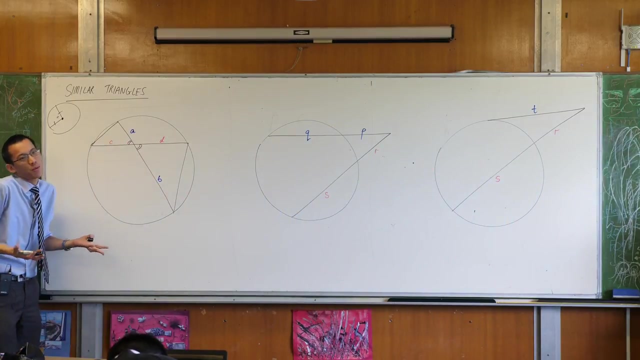 me one Vertically opposite. so right in here you have these two being equal. Can someone compare? Think back to your properties. Yeah, go ahead, Russell. Okay, so I've actually not labelled the angles at the moment, I've just got lengths This. 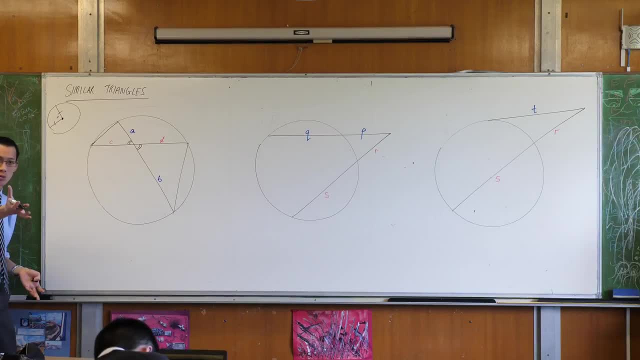 is actually the property is about lengths, but tell me the property that you would use to prove that angles are equal. Yeah, Very good. So, for example, see this arc down here which is unlabeled. You've got this guy and this guy both standing on that arc. You could make the same argument talking. 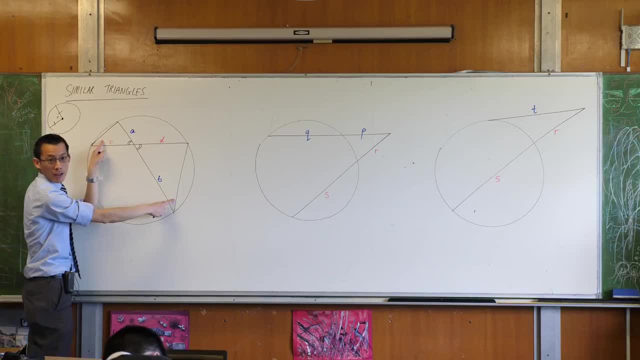 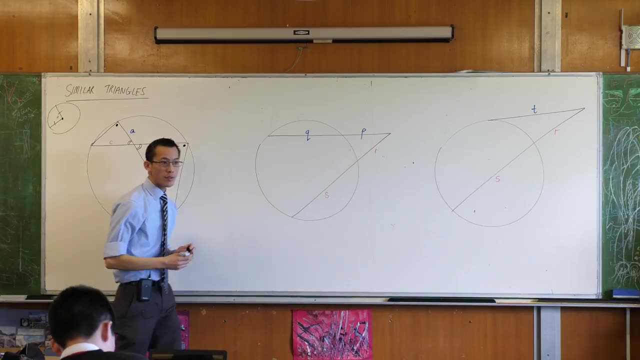 this arc at the top. these two are standing on that arc. Does that make sense? Doesn't matter which one, Let's just do this one over here. So I will leave the formal part of this for later, because it's really not that big a deal. You guys know how to prove similar triangles very easily. 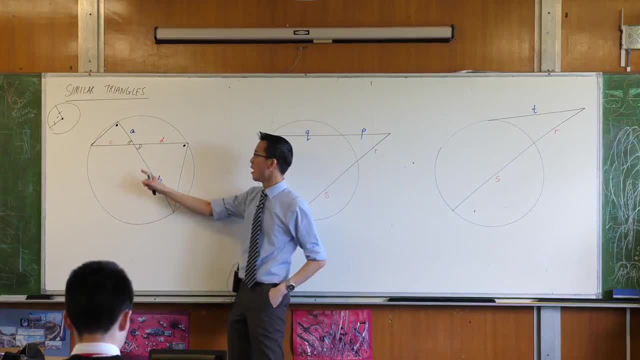 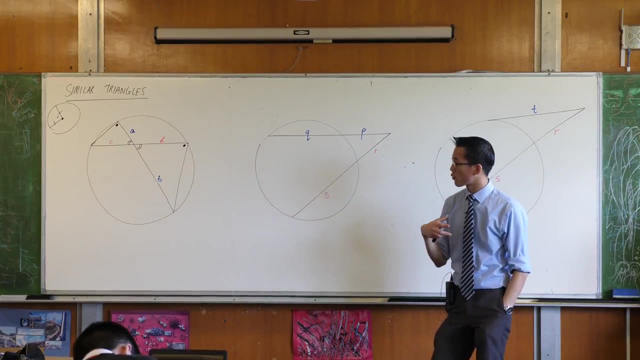 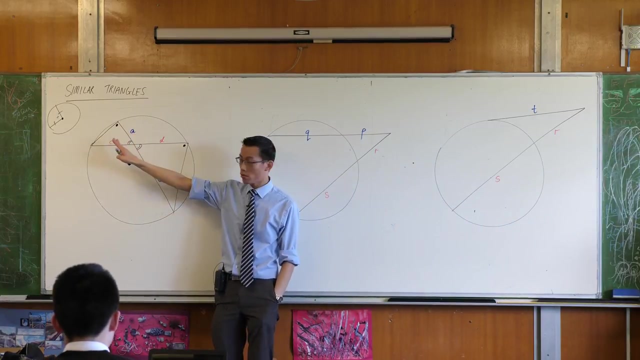 But you've got a pair of equal angles there, a pair of equal angles there. they're equiangular. I'm done So. now the interesting part comes from the relationships between these sides. I want you to have a look at the sides up in this small triangle and which sides they correspond. 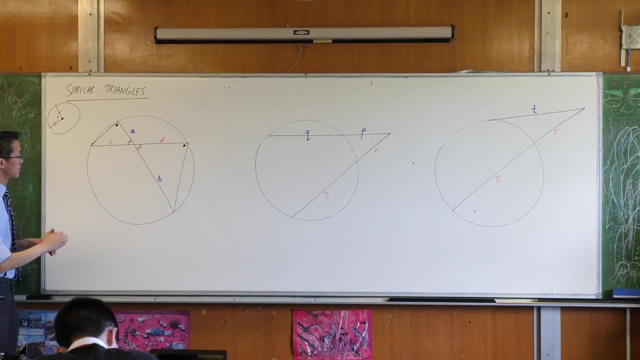 to in this larger triangle. So, for instance, side A in this triangle is the one between the dot and the double line angle there. So which side in the other triangle corresponds to A? It's D. right, You can see, they're both. 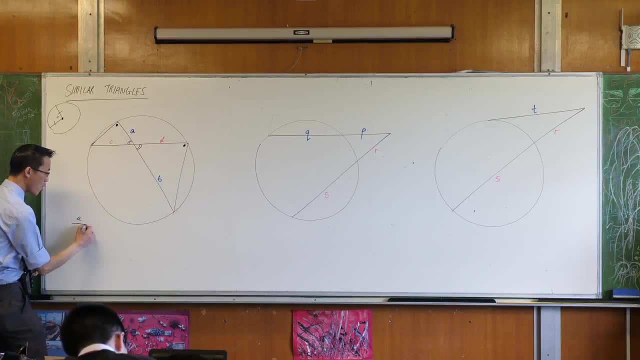 bracketed by those two angles. So A over something is going to equal to D over something. So there are the sorry. what did I just say? No, it's the other way around That way. I never did So. these two. 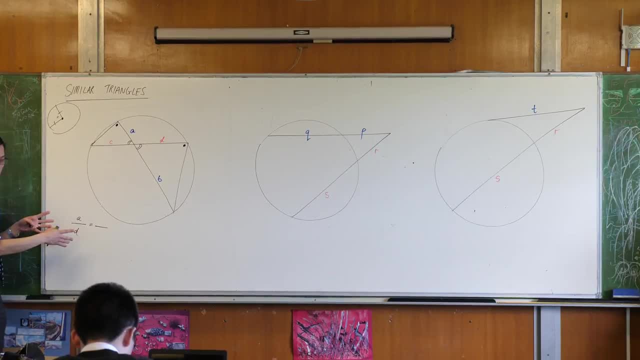 sides correspond to each other. That's the ratio of those corresponding sides. So that only leaves the other ones, which are: let's see, here I'm going to have. this is the small triangle, this is the B triangle, So out of C. 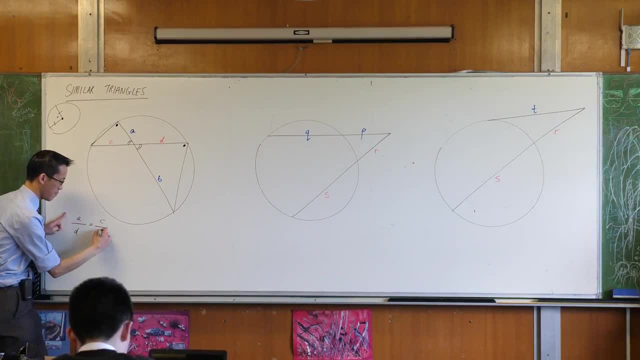 and D, which one goes on top C And then B down here. Does that make sense? And my reason, of course, is corresponding sides in similar triangles are in the same ratio. Now, this is true, but an even nicer way to say it is to: 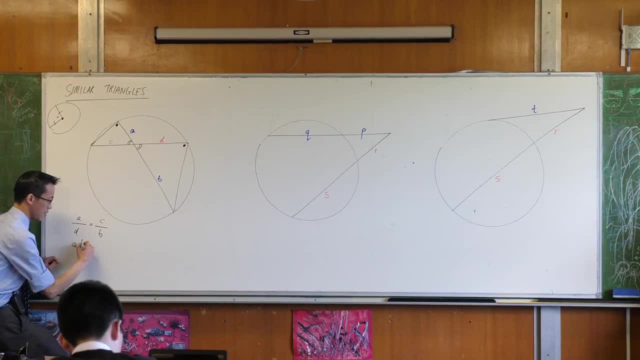 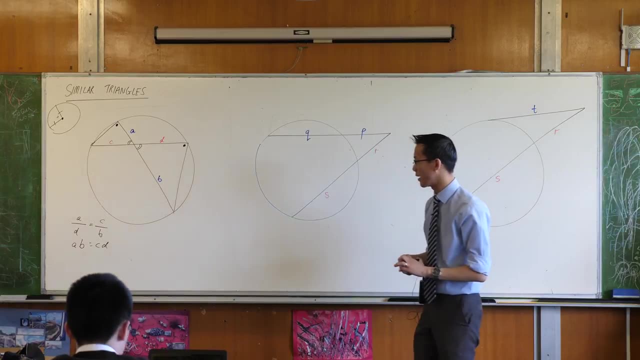 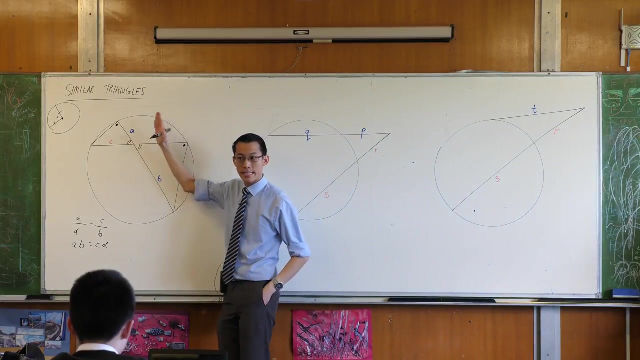 cross, multiply right, And you get AB equals to CD. Isn't that a nice, incredibly simple relationship between all of those four different lengths? So how would we say this? Here comes the wording for this right. You remember we said these are intersecting.